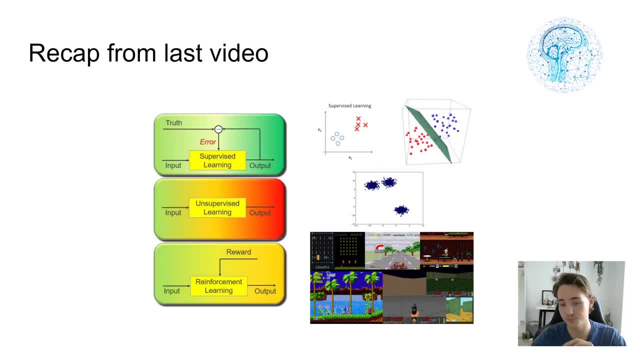 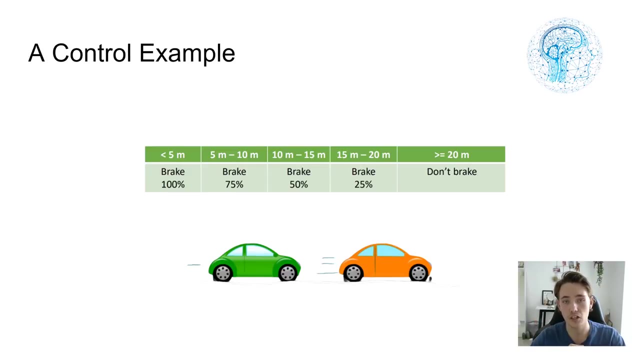 um some like act. it takes some action um from like the inputs that the reinforcement agent is is given and then it gets rewards for for like how good it has performed by doing that action in in the environment. so to go back to this video, we're talking about like fuzzy logic and control. 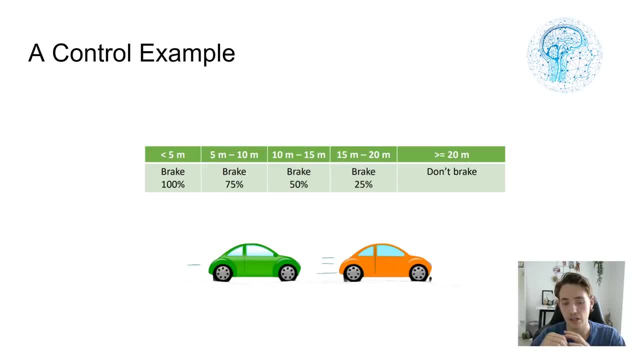 so let's start with a control example here, where we have um a car driving and then it is like measuring the distance to the car in front of it and then if it, if it comes closer to the car in front of it, it will like slow down or like hit the. 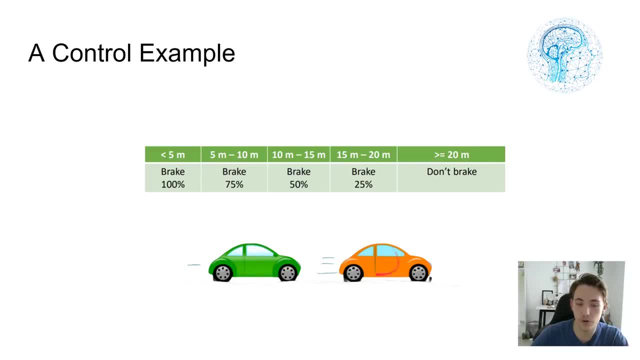 brake. so in this case here we can see like the green car is going up to the orange car here and if it's under five meters and to it to the orange car here, it will just like break 100. so we'll just stand on the on the break and break 100. 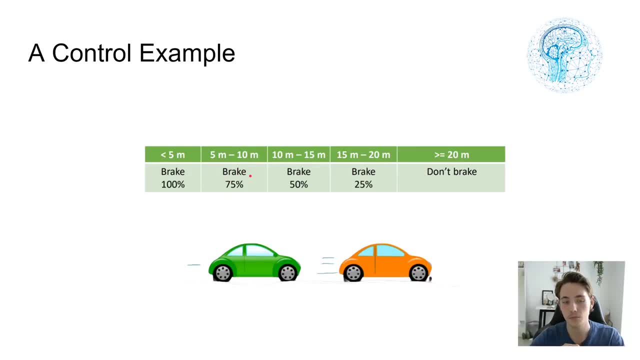 and, uh, 5 and 10 meters to the car in front of us. we're just, we're only hitting the brake with 75, and then we just keep doing the same in smaller steps until we're like more than 20 meters away from the from the car in front of us, and then 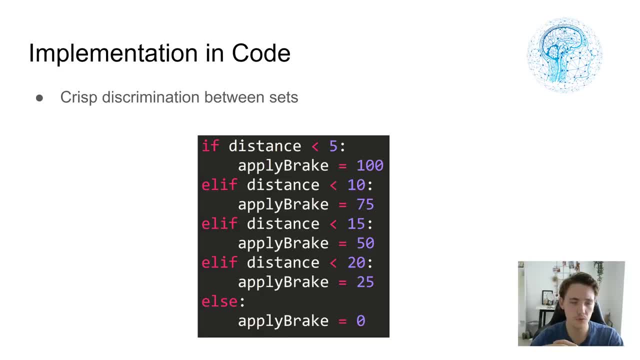 we, then we don't break. so if we want to control, uh, implement this kind of controller in in our code, we can just do it with an like a switch statement or a state machine where we, where we are in different kind of states. so this is called. 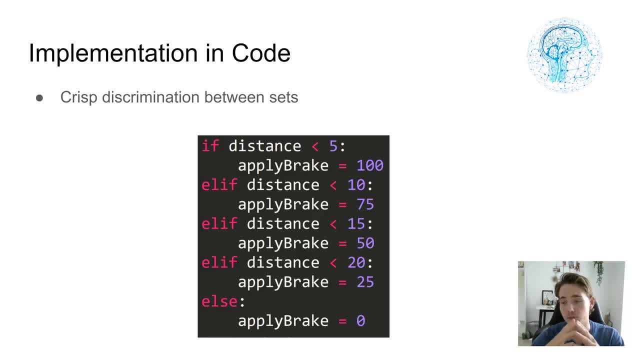 the crisp discrimination between sets, because we have like some rules or that is set up and if something, if something is true and then do something else. so in this case, if we just implemented the, the rules we set up here, so if the distance is less than five we just apply the break like 100, we apply the reply 100 to. 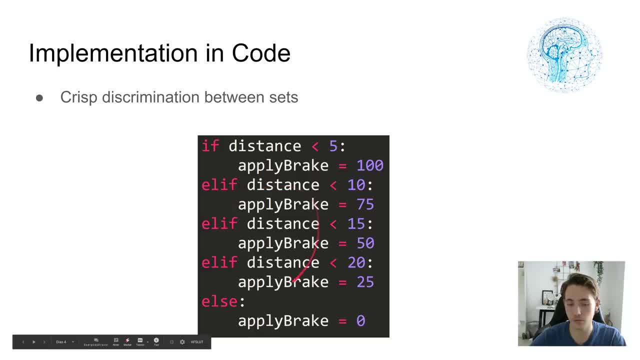 the break and then we just keep doing the same here with the other other states that it could be in. but the problem with this is that it is like it is either like apply to break 100 or apply to break um 75, so it's more like a crisp. 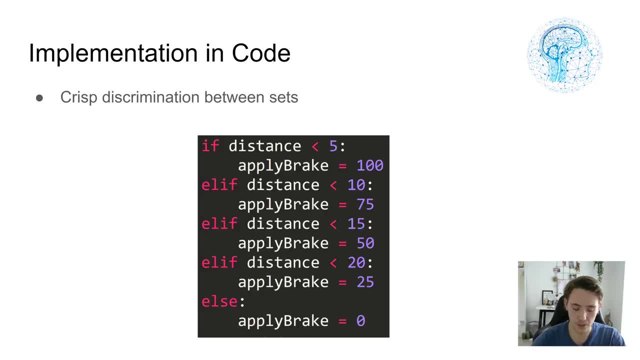 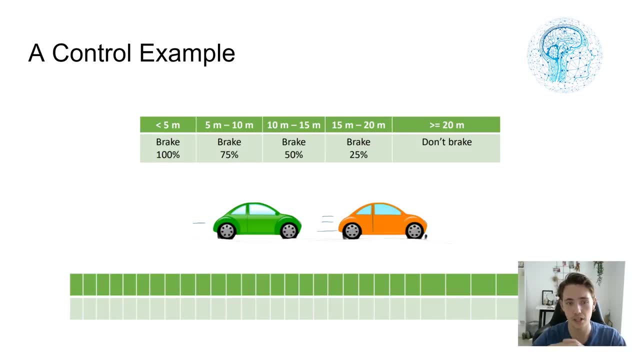 discrimination between the sets. so it's it's either one of them, where, where, like in fuzzy logic which we're going to talk about in in in later in this video, it's. it's more like it can be like um, some of some of both. so it can be like it should break like 75, but also like 100. 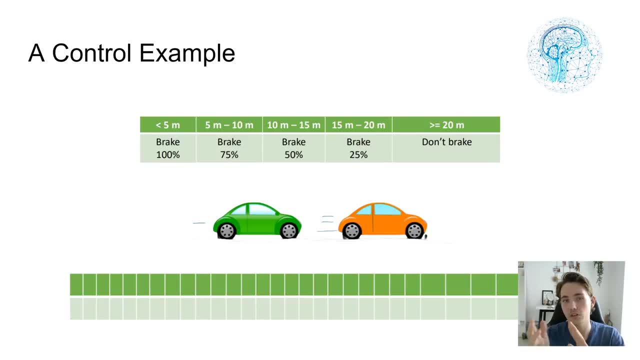 so it's not like crisp, so it's not like either one of them like. so it's not like, uh, boolean logic where you have true or false, but more like you can have some, some more steps between those, those rules that you set up. so the control example here is just like: how can we like, do it more? 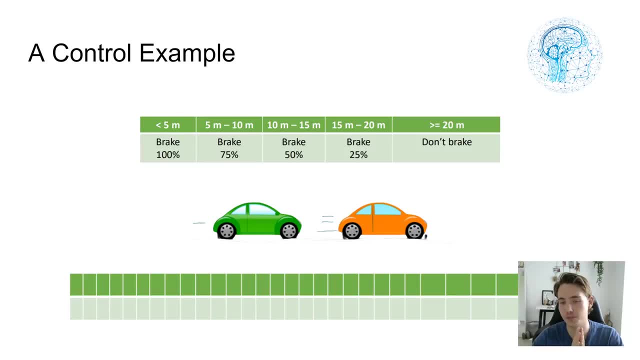 like it continues, instead of these discrete crisp sets that we're just dividing in. so we could actually just make more steps. so instead of like having five to ten meters here, we could have like five to six meters, but it will still be crisp set, even though we just 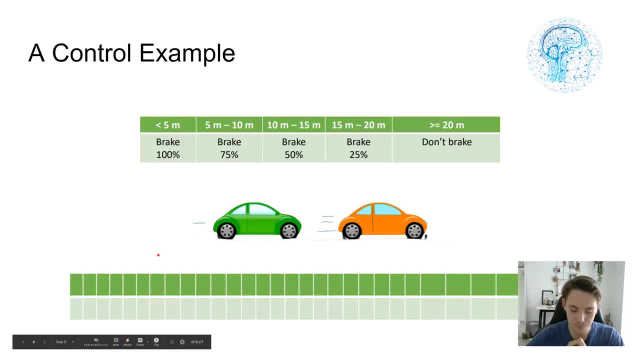 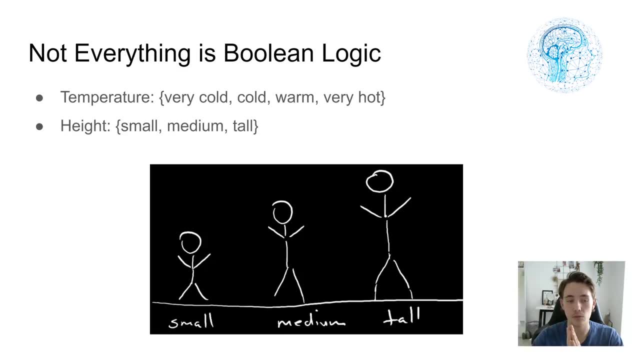 divide it into like smaller rules or like smaller states down here. so the solution to this is that not everything is boolean logic, where, like boolean logic, is either a zero or a one and if we want to like apply some control system, it's not really like, it's not good. 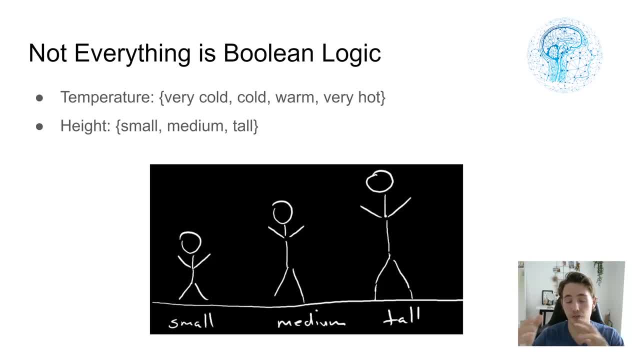 and it won't be continuous. so if you're, for example, in a car and you just if you're in five meters to the car, to the car in front of you, you'll just step on a break and it will not be like if you're five meters, then 75 percent, I apply 75 percent of the break, and if you're like just 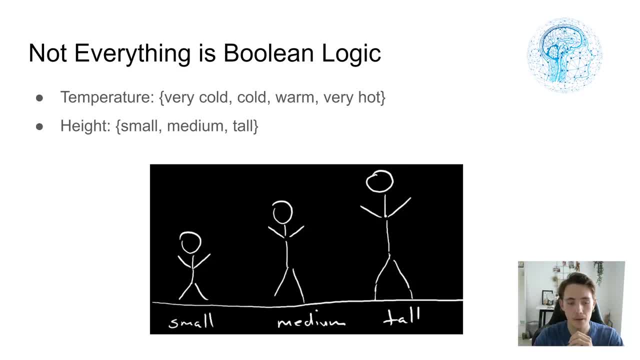 going one meter behind you only apply like 50 of the break, so it's not really like. everything is not boolean logic, and especially when, when we're talking about like reality or just like stuff like that. so an example here is also like temperature, when we want to like divide. 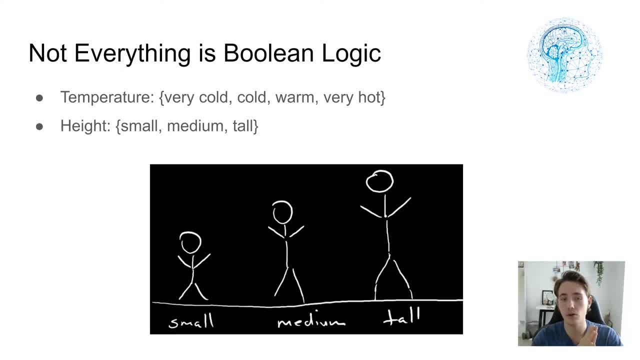 something into temperature, so it could. it can either be like very cold, cold, warm or very hot. or let's say like, for example, here we have the small, medium and tall, and on the picture here we have a person that is either small, medium or tall. and then let's say, for example, we had a 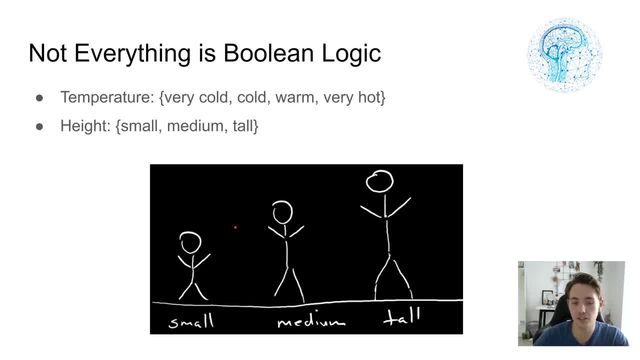 person here in the middle. so with boolean logic we can really say that this person in the middle here is like medium, small or small, medium. so if we use boolean logic for this, it can either be like this person is either small or medium. but when we're using fuzzy logic, we can actually say that. 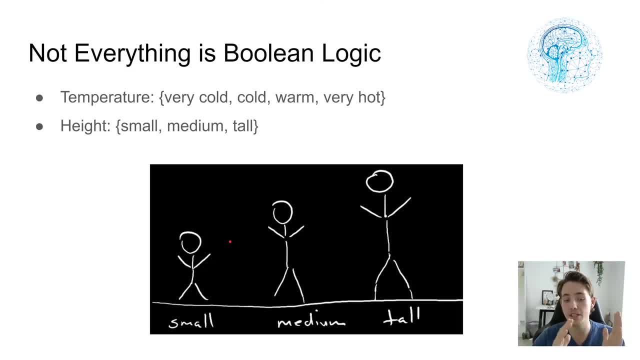 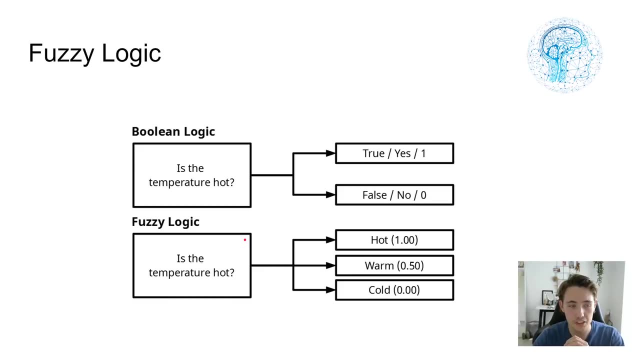 that this person in the middle here like a step between our rules. it can also like be a small medium step, so we just like kind of divide our, our program into smaller and more like continuous steps. so it's- uh, it takes us further here to like fuzzy logic and the introduction to fuzzy logic. we're 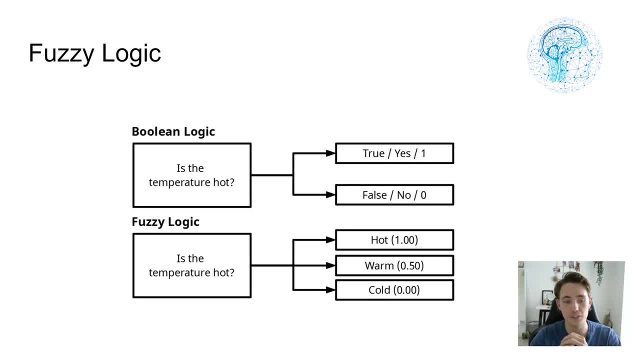 also going to talk about a fuzzy logic more in depth in in the next video where we're going to like um, talk about like the fuzzy logic controller and how he element in the in the fuzzy controller works. so this is just more to like, compare, like we are normally used to, to boolean logic where it can either be like false or true. so in this case, 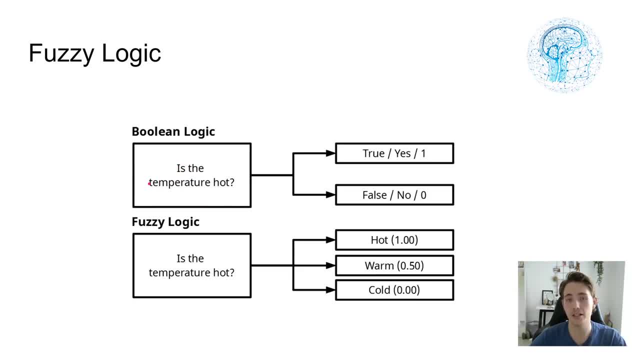 here we say that is the temperature hot, and we can either say like yes, it's hot or no, it's not hot. but with fuzzy logic we can ask the same question here again, and is the temperature hot? and then we can say like yes, it is, it is 100 hot. or we can say like it is not, oh, it's only like 50. 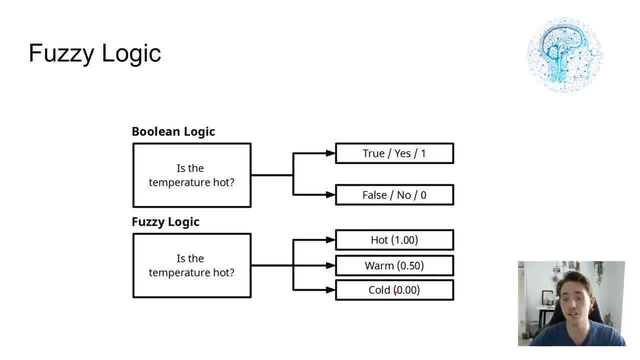 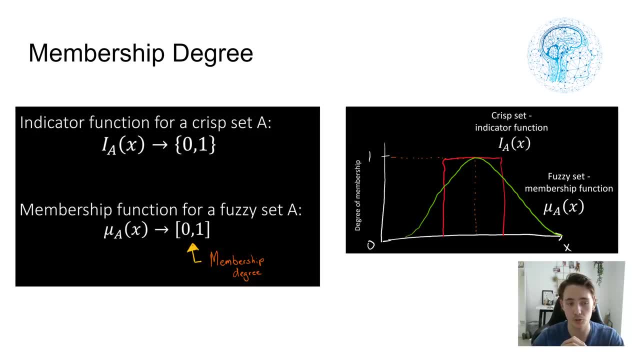 percent hot, or or it's, it's cold. so we divide them into like smaller steps and if we go to the next slide here we can see that we define fuzzy logic with a membership degree or a membership function. so, like for a crisp set, here for boolean logic we have, we have either like only zero or or one. 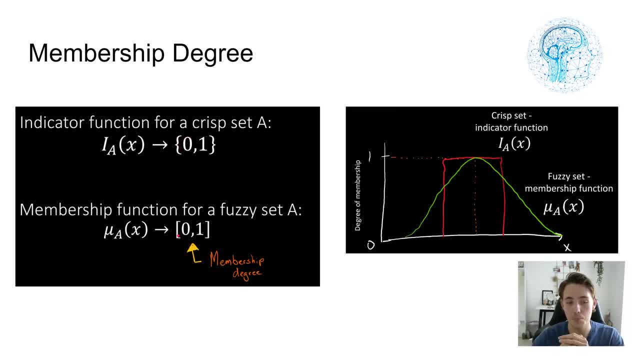 where, where, in fuzzy logic, we have something called a membership function for our set. so um, it's a. this is our membership function here for the fuzzies at a where. this is the membership degree. so the membership degree is like: it's not one or zero, it's it's a number between zero and one. so 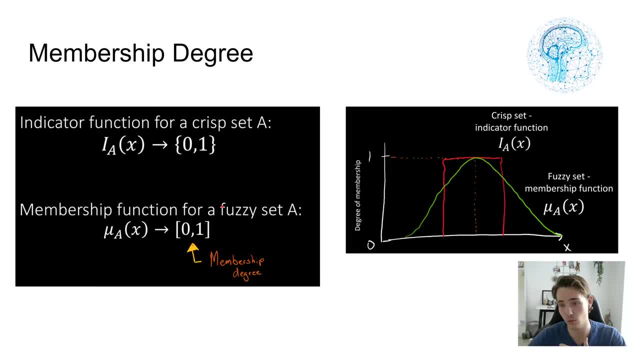 it's like smaller steps between those two numbers, instead of just one of them, and, and. and this correlates to to the graph over here where we have like the degree of membership up here on the, on the y-axis, and then we can see, like the red graph here, like the red graph here is the crib set, chris set. 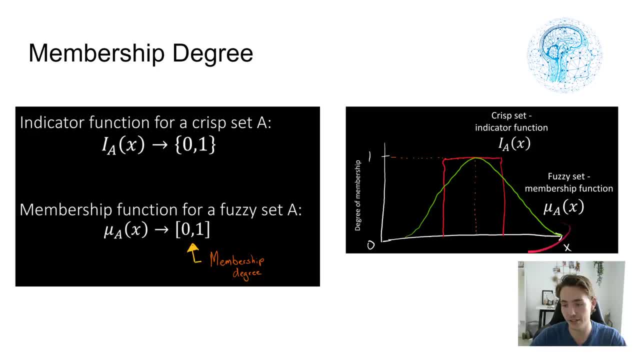 indicator function where if we go on here on the x-axis we can see that if something uh occurs, then it is, it is either one or zero. where if we have like our, our membership function here for our fuzzies set, we can have like um, actually we can have arbitrary, like forms of of grabs and 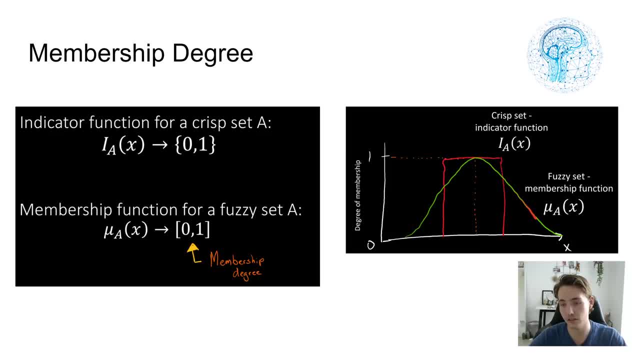 lines and stuff like that. if we want to, we can also have like have triangles or some other different kind of functions or palominums or stuff like that, but in this case here we just have like a gaussian- uh, gaussian graph representation here um where we have like, where we have like um our 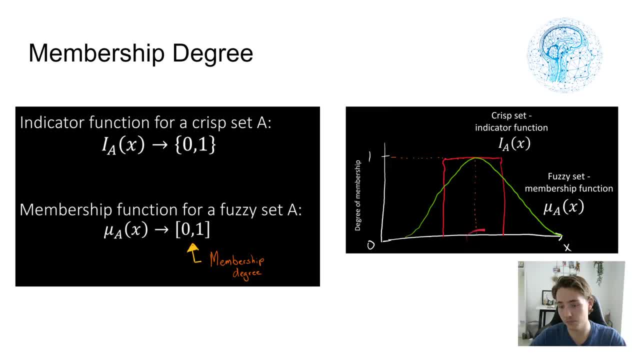 degrees of membership, like they're increasing here. for example, if we had um the like, the cold here and we will say, like here it's, it's very cold, but then we are like we're like um, going towards a very cold, like cold here, so we can have like if. if it was the same as the persons 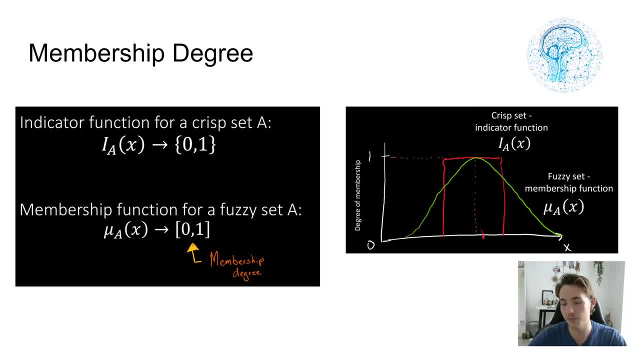 we just talked about, where we have like um small here and then medium here. then we can have like small, medium here, which indicates of the degree of membership, like, let's say, 0.5, which will indicate like a small, medium person, where if you have like a crisp set function, it could either be like a small or or medium. 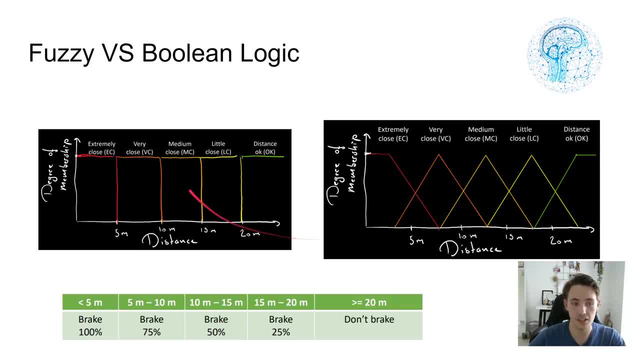 so this is just to compare like fuzzy and boolean logic, where on the left here we can say that if we go back to our car example again here, where we, where we like, divided our problem or our control problem into into these steps here and we try to 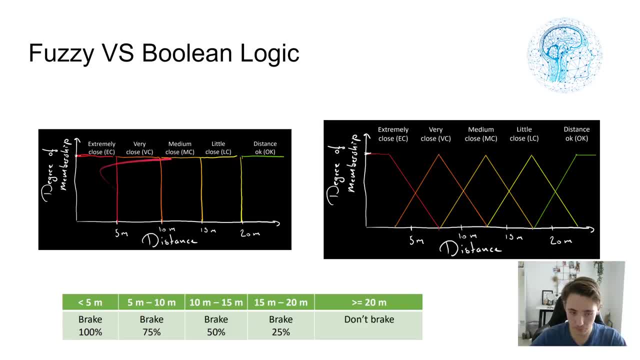 to draw a membership function, um, like a graph over here where we have the degree of membership up. here we can either be like extremely close, very close, medium close, little close, or like the distance can be okay and we don't need to apply the break, and then we have our our meters. 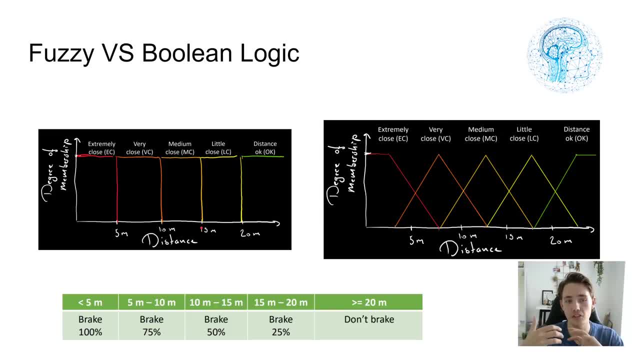 here down on the x-axis, where if we use fuzzy logic instead of boolean and logic for this control, we can see like with these triangles over here, we can then have our, our, um, our fuzzy logic function and like these triangles here where we can say like we go from extremely close and then 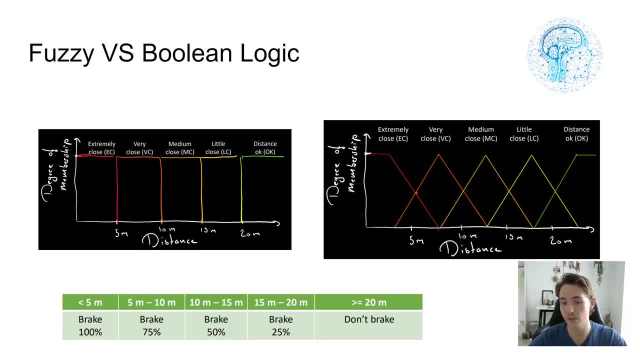 it gets less and less and less, extremely close, until we hit like five meters. and then it gets more like very, very close, but not very close, because it will only be 100. very close when, when we have the degree of membership here at one. so, and then again it will be. 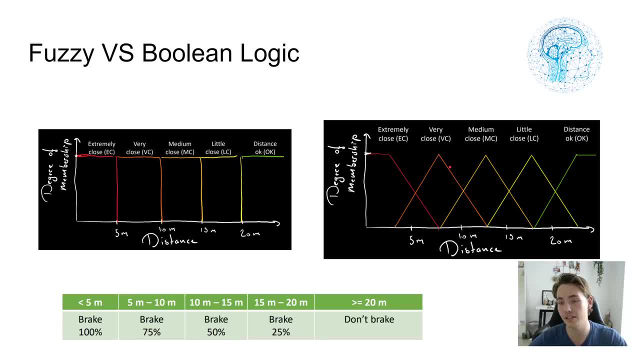 less and less and less close to very close and then like closer to medium, close. i just switched, so this isn't like more to into like divide, our, our like control problem into smaller tasks and then we don't. we don't only have, it can either be false or true, but we can have, like, for example, 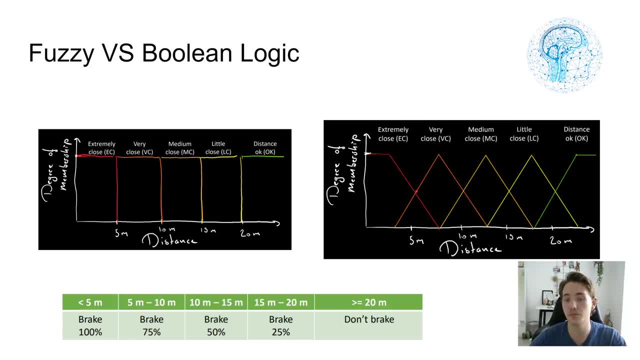 it's 20, it's here, it's- let's say it's it's 15, 50, 50 extremely close and 50 very close. and then we go over here and then we say like now it's 60 close and only 40 percent extremely close. so we have like some, some, some. 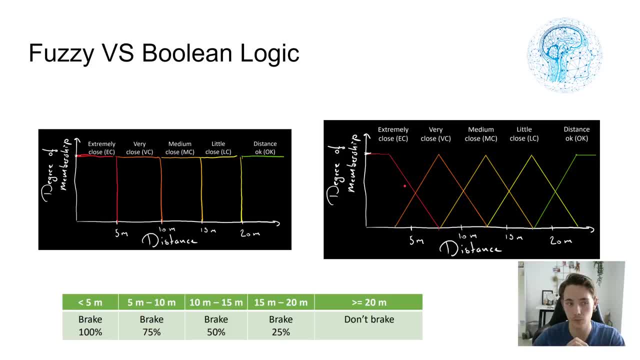 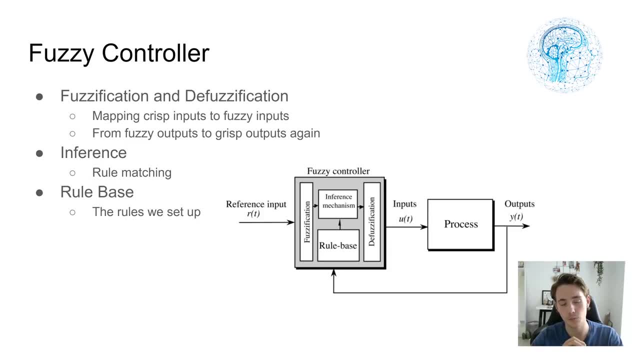 steps in between or are like crisper steps with with fuzzy logic. so when we, when we're using our fuzzy logic, we often use it like as a, we can use them as a fuzzy logic controller. where we're going to like- like, for example, in the example we had with the cars- we're going to implement a controller that can. 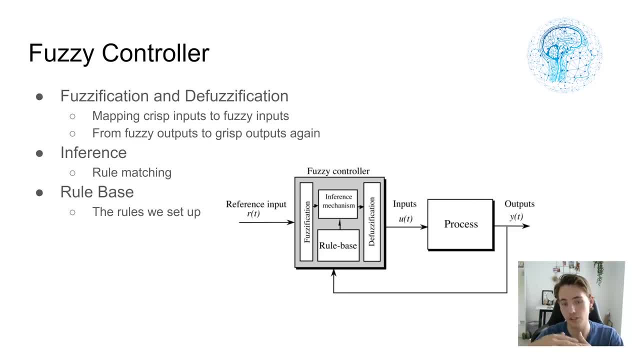 that can break when we're like, when we're going like towards another car in front of us and then inside of our fuzzy controller. here, first of all, we have a reference input that comes into our controller and in this case it could be, for example, like the sensor- the sensor values fraud for measuring the distance. 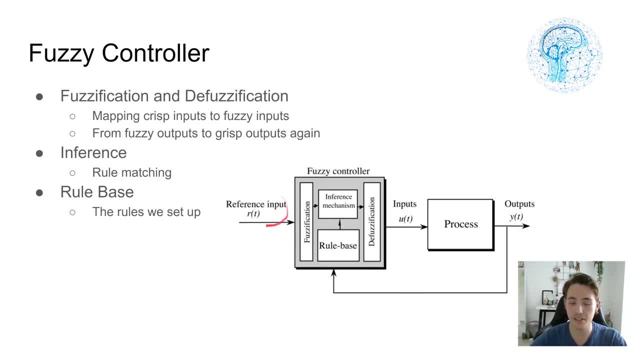 to the car in front of us. and then when we get that distance, here we fuzzy, we use the fuzzication here to like to like: get from a crisp set- it will be a crisp input- here we get into our fuzz controller and then with our fuzzification, here we like, we convert that, that crisp input, to a to a. 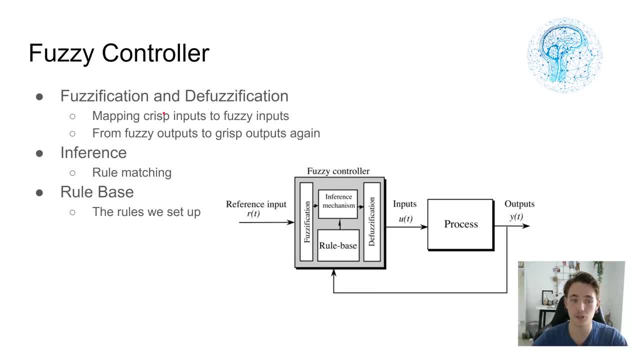 fuzzy input. so, as I said up here, first we're mapping the crisp input to a fuzzy input and then we have like some inference mechanism here. that is like rule matching. so for a fuzz control we have to set up some rules as like, let's say like very close, close, a far away and distance is okay and stuff like that. 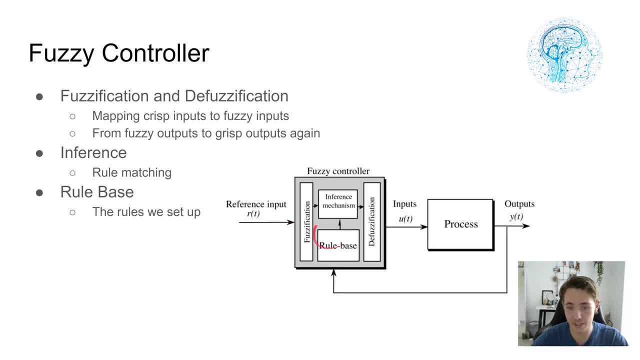 so and then we have the rule base here. that is an inferring with like, like. the rule base here is where we, where we like, set up our rules and then, in our inference, is where we match those rules to the fussy fussy input we get here. 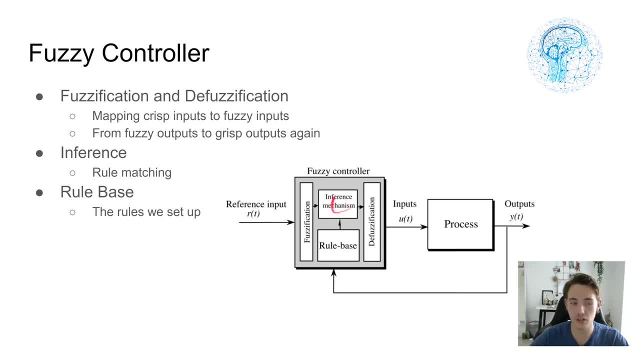 from our crisp set and then when everything is done and we have matched the rules we have set up, we can go back again and defuzzificate our output from the controller here. because when we need to apply our input to the process here or to the car when we have to hit the brake, then we need a crisp output again. 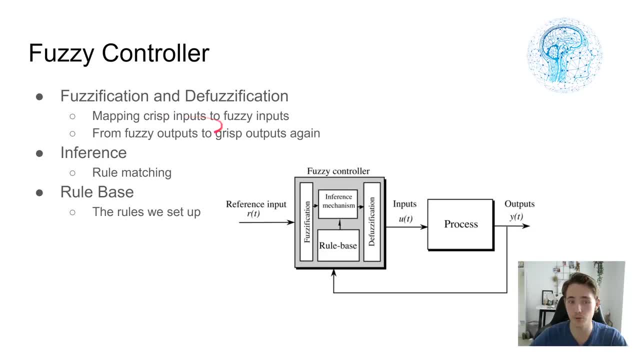 so in the defix case in here we have to like get our fuzz inputs to crisp outputs again and then we can apply that crisp output to uh, to our brake or another process that we want to control, and then we feed back that output here again to our fuzz controller. um, for for like the next. 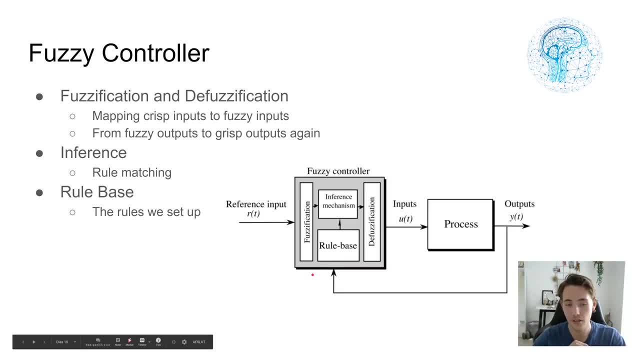 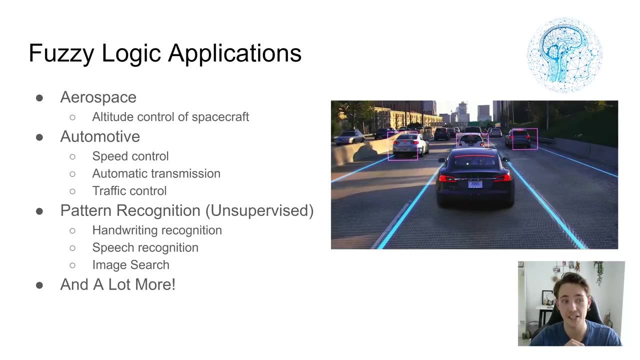 calculation. so we'll calculate some, some, some kind of error and then use that, that error, in in terms of like the inputs and outputs for our fuzzilogic controller. so on the last slide here i'm just going to go over like some, some different kind of applications that we can use fuzzilogic. 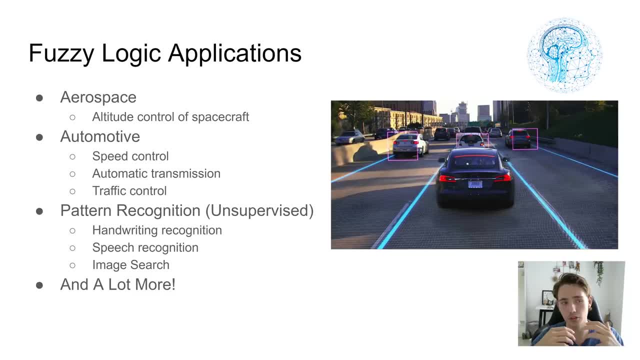 for because it's a very used. it's a very used concept inside, like a control engineering stuff like that, because it is, it is kind of it is kind of easy to set up and then in the next video we're going to talk more about like how, how these um fuzzy controller and 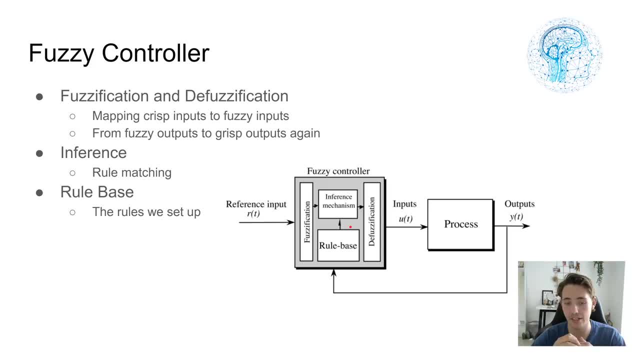 different kind of elements inside the fuzz controller, like how they work and how we can go from a crisp input to a fuzz input and then, um, do some calculations, stuff like that inside and then, and then defuzzificate our crisp input, a crisp output again, to like a frosty output again. 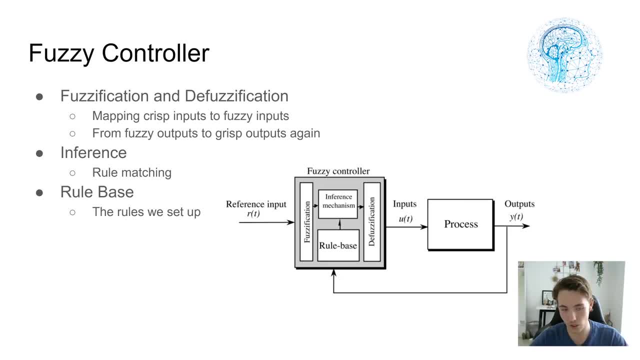 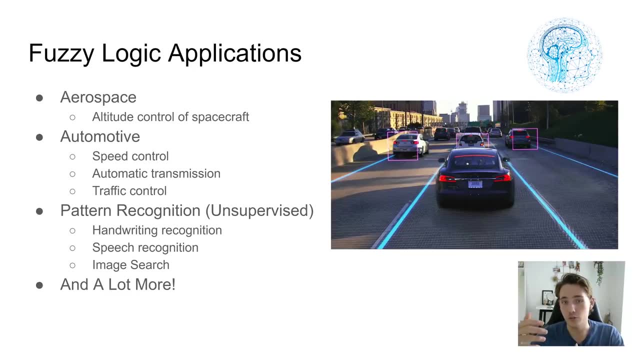 to a crisp output that we didn't can apply to to our process. so we're going to talk about that in the next video. but here here are some different kind of examples and where we can use fuzzilogic and for example, in aerospace we can use fuzzilogic to control, like, the altitude of the spacecraft, which is like kind. 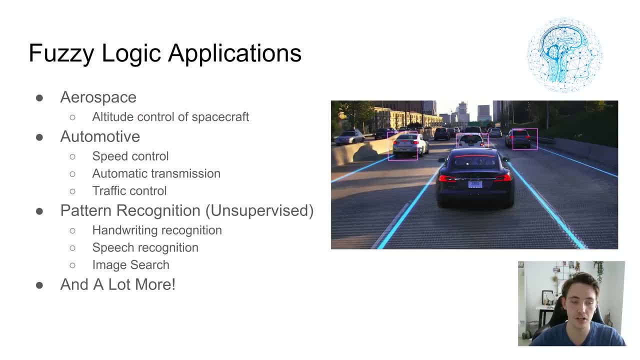 of the same as we did with the, with the brakes here to to the car in front of us, and we can also use it in automotive applications for speed control, automatic transmission, like when you're shifting, shifting gears and stuff like that. so we don't really like, just want to be like either did. 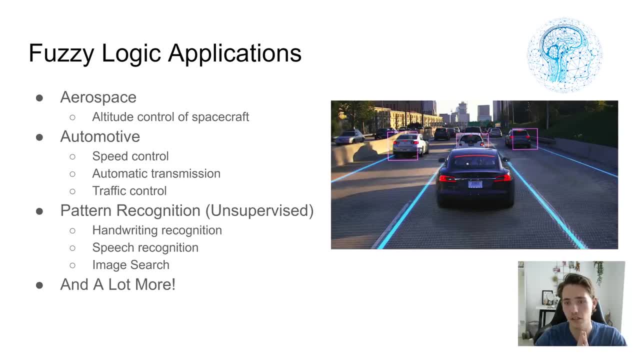 skier and and stuff like that. so we want to have those like more smooth and continuous and transmissions between the gears, but also like for for traffic control. it's also uh pretty used in for, let's say like in in power recognition if we have some kind of super unsupervised um problem. 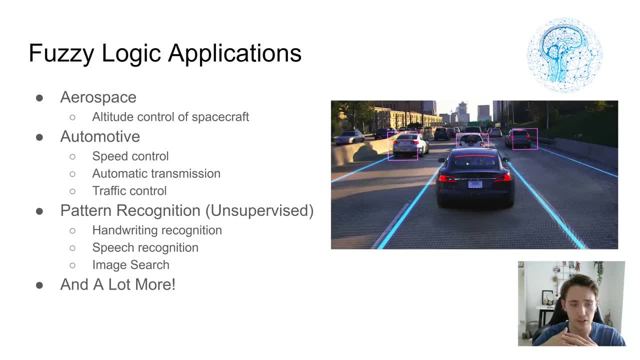 that we want to, that we want to like get something out of and we want to try train our model to to learn patterns in in the data. so it is. it's used for some like handwriting recognition problems and also like speech and recognition and image search. so we're going to talk about more that in in the in in later videos. 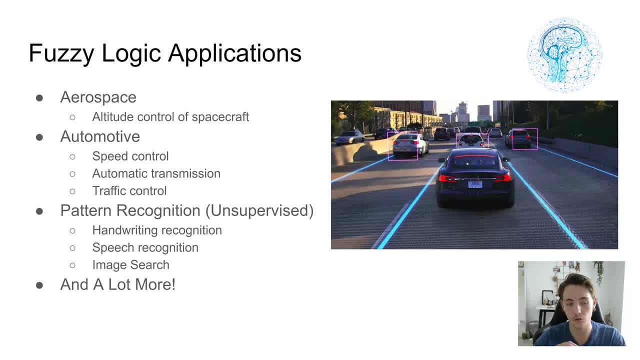 as well when we're going to use um, reinforcement learning and going more in depth with that. but it is also used for a lot more that you can look up in the internet. so it's a very used controller and and like. it's a very practical controller because let's say, for example, like p pids or like: 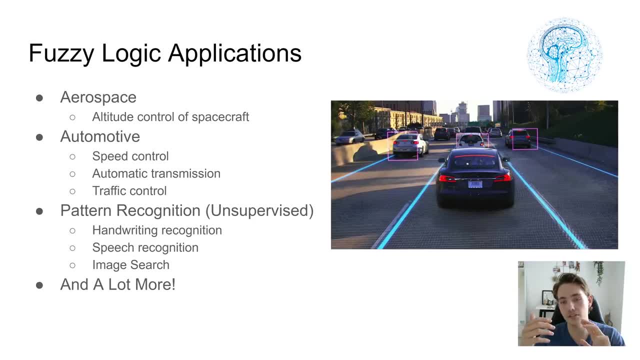 it's like the classic controllers we have. they are not really easy to implement in in in practice, like, for example, with our fuzzy logic controllers where where, like those, they're really um easy to implement in code- and we're also going to do that in later videos- where there's a library for, for a 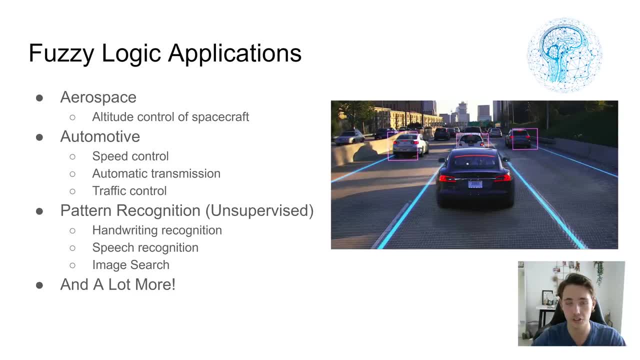 c++ that we can just use for creating our fuzzy logic controller and then use it for for some practical problem then that we set up. so that's it for each of you guys. remember to subscribe notification on your video and also like this video if you enjoyed the content and you want. 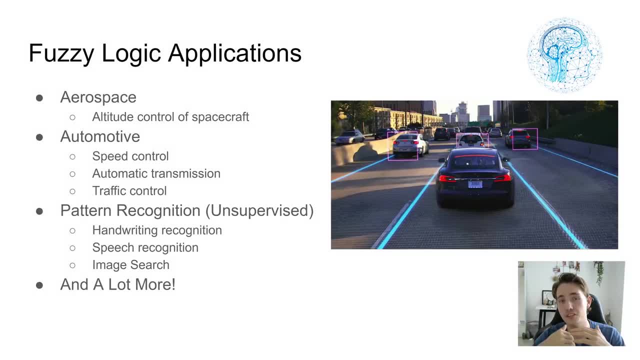 more in the future. currently i'm also doing a computer vision tutorial and also a algorithm and data structure tutorial. so if you're interested in that, you can go check them out. i'll link to one of them up here and then, if you, if you want to, you can go check them out, or else i'll just see. 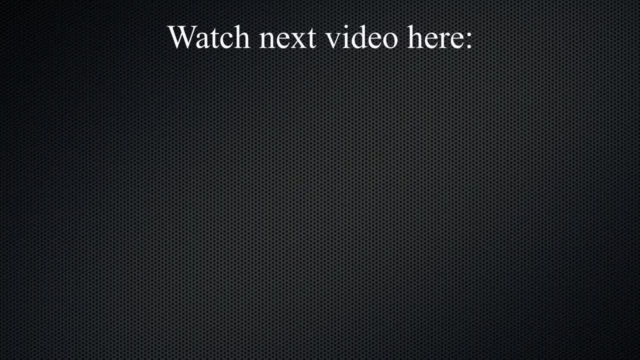 you in the next video, guys. bye for now, you.